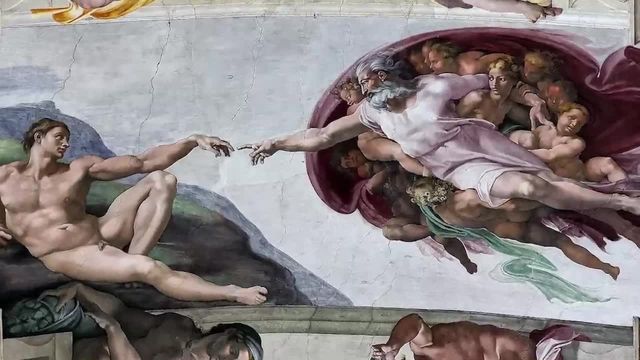 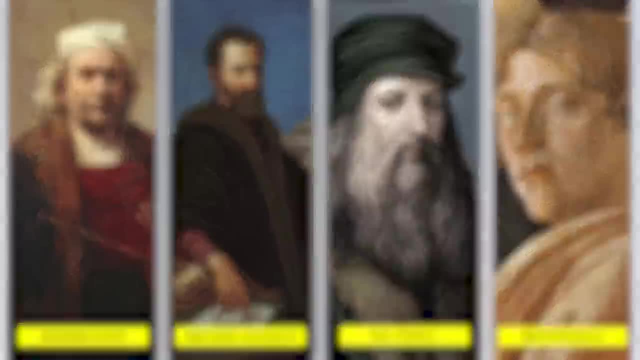 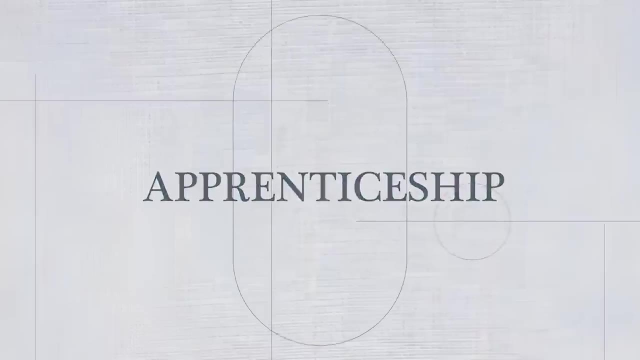 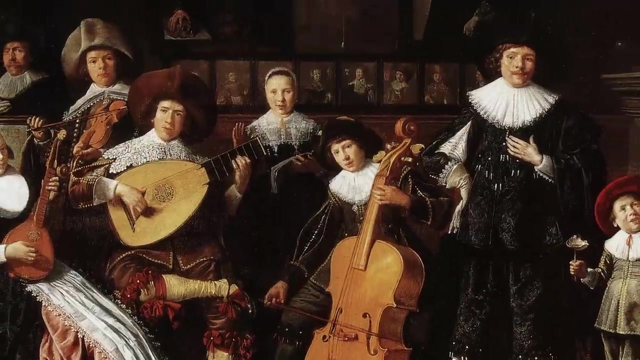 into legends. They were definitely talented, but the renaissance period was defined by an apprenticeship process that systematically churned out artists that we admire till today. Apprentices often entered workshops at a young age, sometimes before they turned 10. They became part of an artistic lineage, frequently connected through familial or marital ties. 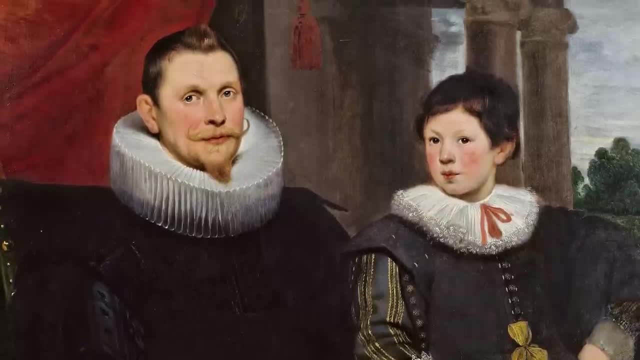 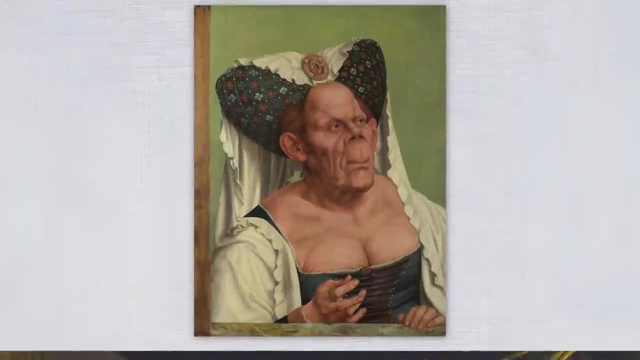 This was prevalent in the art world and likely helped ensure a steady income when sons assumed their father's roles. Pursuing art as a career was often a result of it being a family trade with talent. occasionally taking a back seat, Overseeing the family was often a part of the art. as they pursued art as a career, But sometimes the 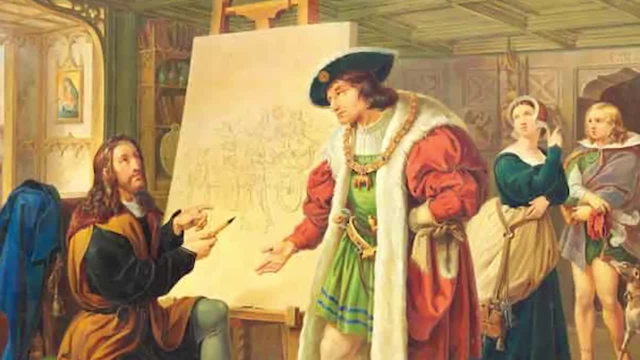 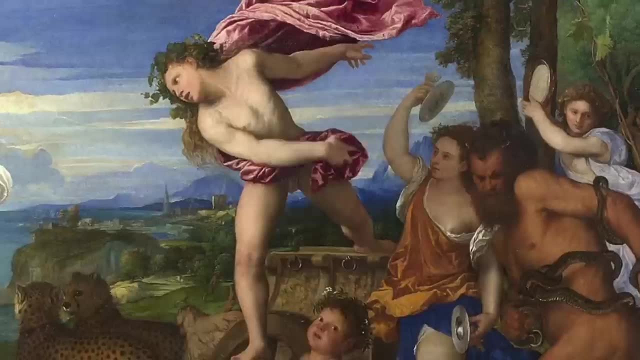 art was also just a part of the family, But sometimes the art was also a part of the family and workshop was the master, who possessed both artistic expertise and keen business acumen. as the apprentice and master worked together, the apprentice learned the craft and contributed to the creation of 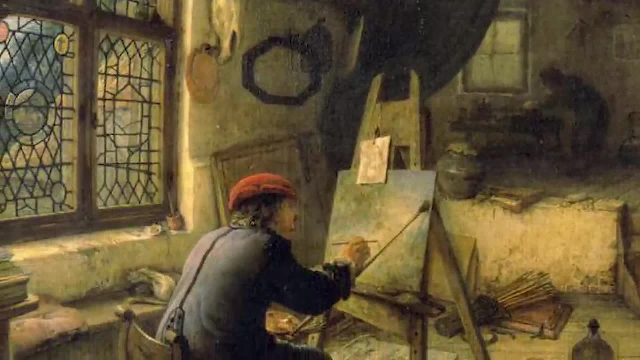 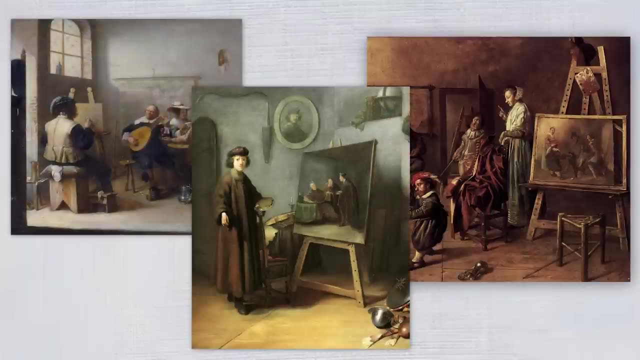 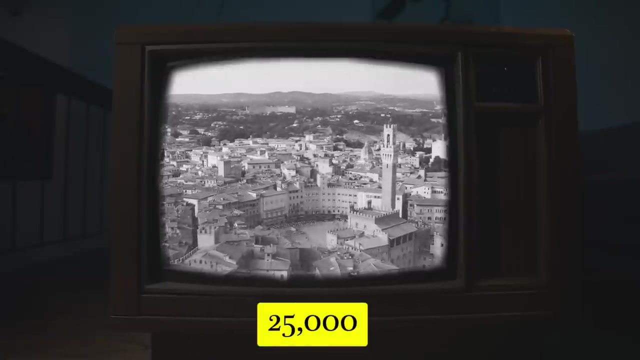 commissioned artwork, and there was certainly no shortage of aspiring young artists prepared to dedicate their lives to the craft. numerous workshops, each focusing on a specific facet of art, employed a significant number of individuals in the late 1300s, out of approximately 25,000 residents in Siena. 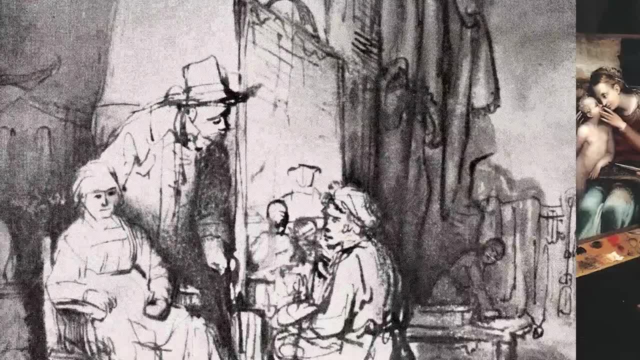 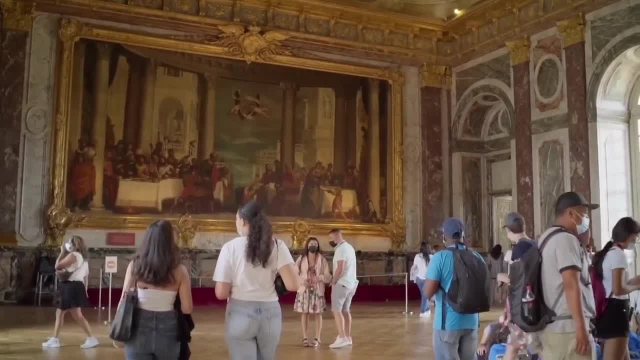 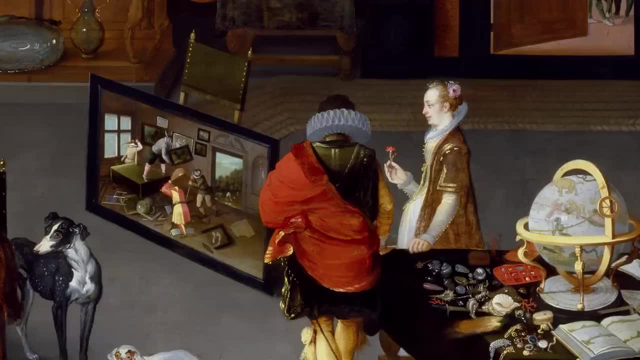 32 or painters and 62 were stonemasons, and by the early 14th century there were nearly 100 painters. today we view fine art as a luxury, something accessible to those with money and connections, but back then, art was something society desired, required and utilized. as a result, a sufficient number of artists 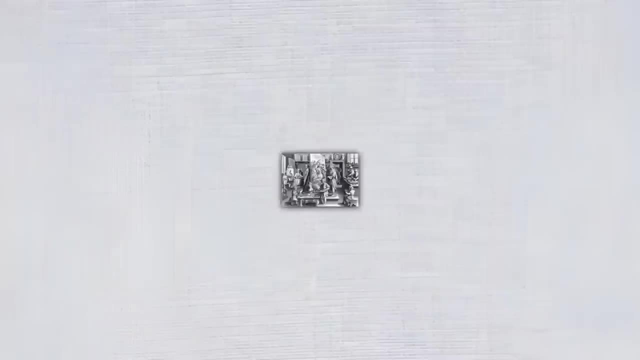 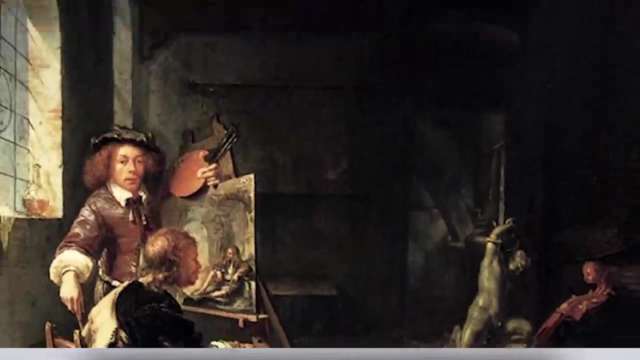 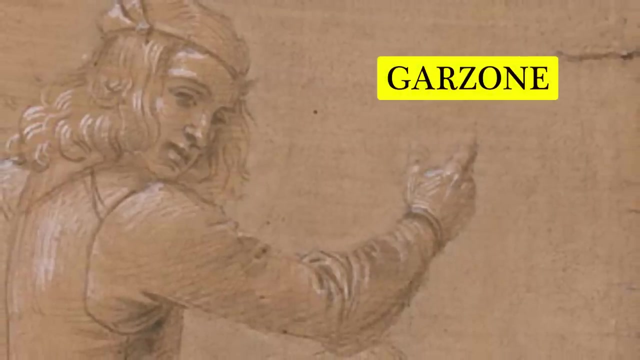 had to be available to meet the substantial demand, and therein came the role of the apprentice. an apprenticeship could last anywhere from a few months, months to several years, with each experience tailored to the ever-changing art market. As an apprentice or garzon, you would become an integral part of the master's household. 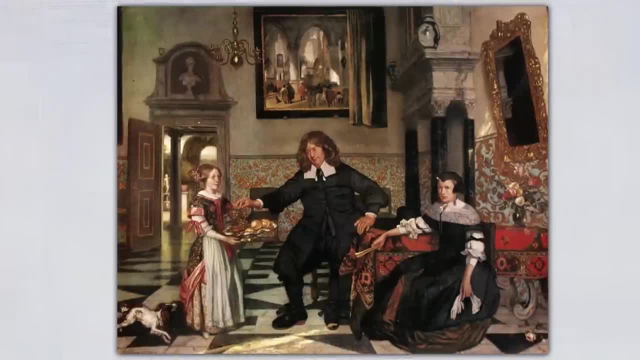 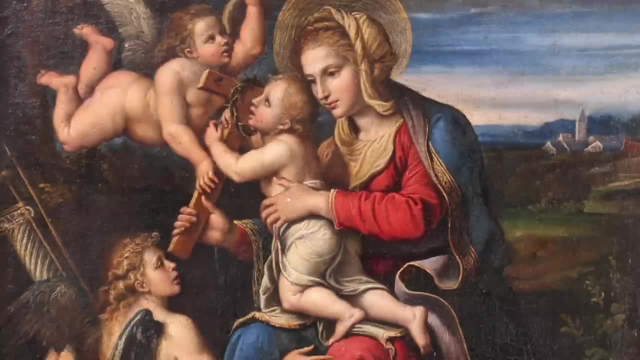 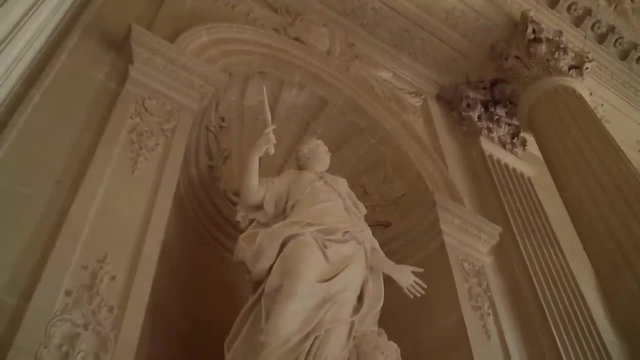 sharing accommodation and meals with the master's family. The apprentice's parents might contribute to their living expenses, but as their skills developed, the master would become responsible for paying their wages. Each workshop varied in structure. When a big project arrived, like a fresco cycle or a series of statues, the workshop would expand. 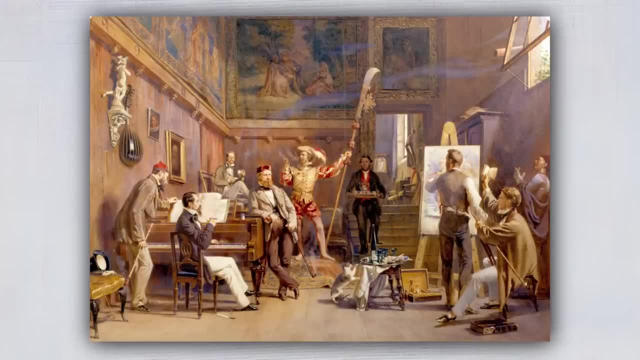 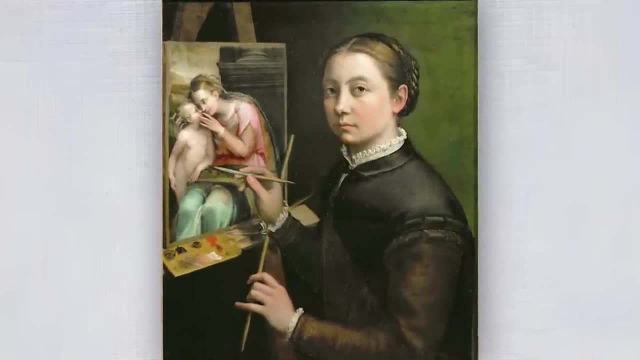 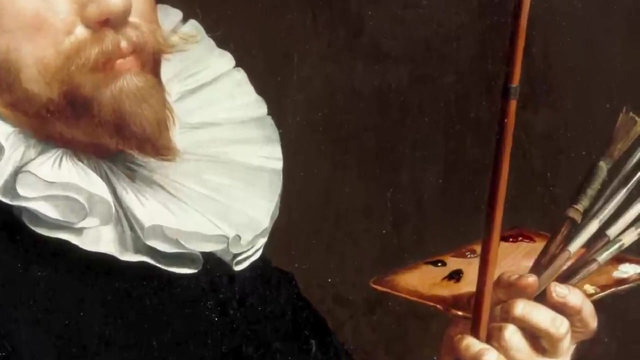 and hire more assistants to manage the additional work. In the beginning, apprentices would start with simpler tasks like preparing panels and grinding pigments. Renaissance artists and their assistants made their own materials from scratch, including paint colors and brushes. This early and enduring knowledge of the material and 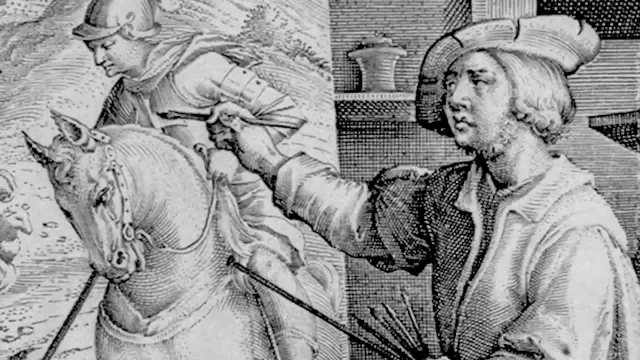 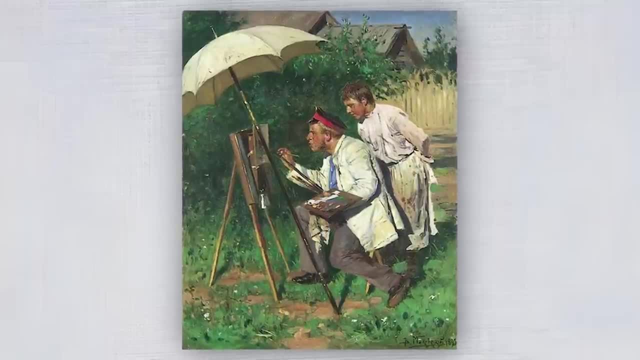 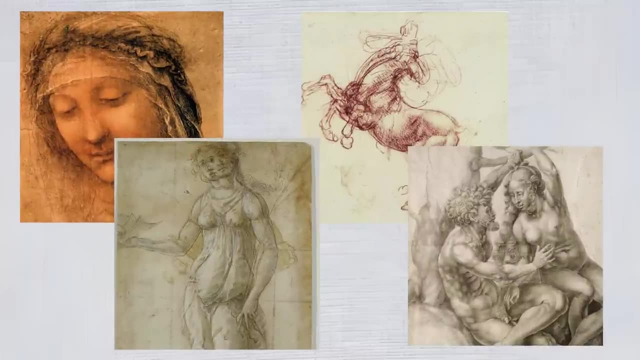 physical aspects of their craft provided the artist with an almost intuitive understanding of the materials. During this time, they would learn to draw by copying their master's drawings or those of other artists. These collections of drawings would serve as both instructional resources and valuable references for future works To further their 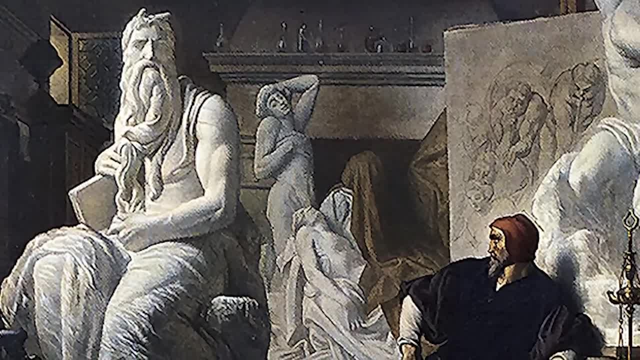 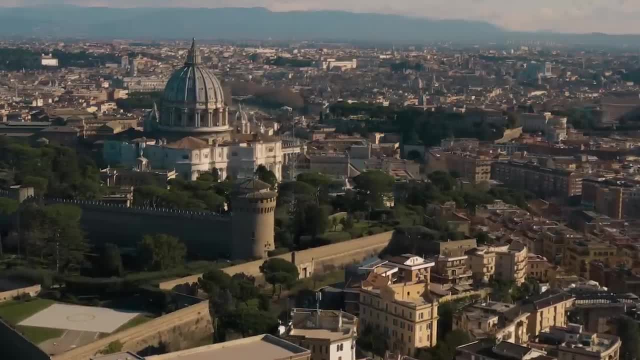 visual education apprentices would study and copy renowned works in their city. You know Michelangelo, right? He replicated Giotto's paintings during his training years. If fortunate apprentices would get the opportunity to travel to cities like Rome to expand their artistic 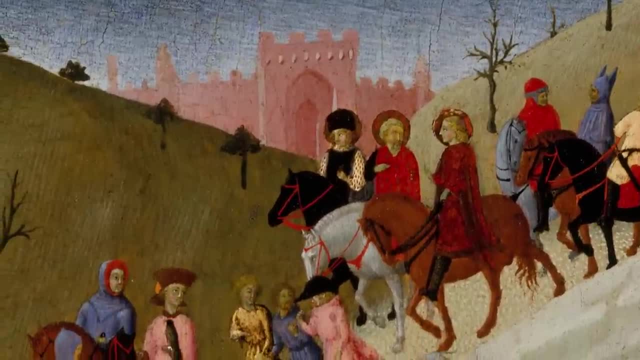 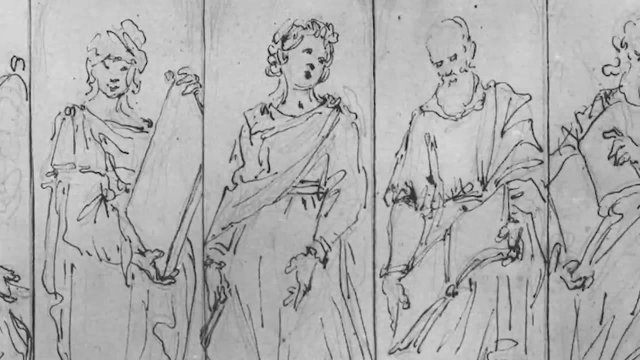 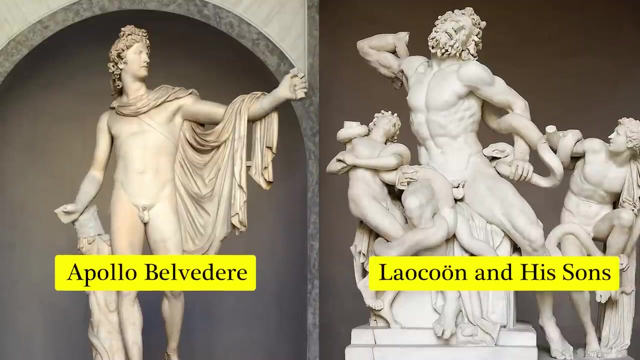 horizons. Accompanying their masters on important commissions would help them gain practical experience and encounter new artistic influences. Apprentices would then progress to drawing from statuettes or casts, primarily using ancient sculptures like these to help bring more naturalism to Renaissance depictions of the human form. Mastering these drawings would 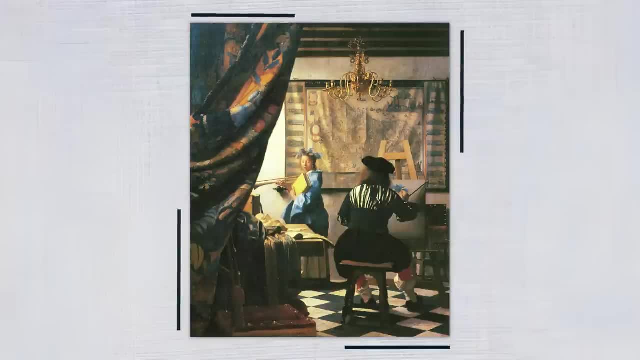 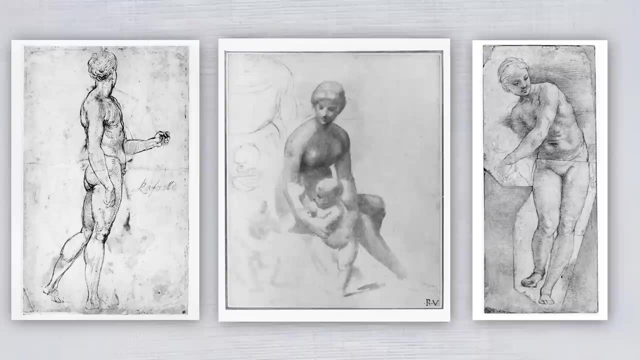 prepare apprentices for the next stage, drawing a live model. Usually, a fellow apprentice would be called to pose for these studies, allowing them to practice their drawing skills. This would help them to practice capturing the human form in various positions. When apprentices advanced to painting, they would typically start by working on less significant 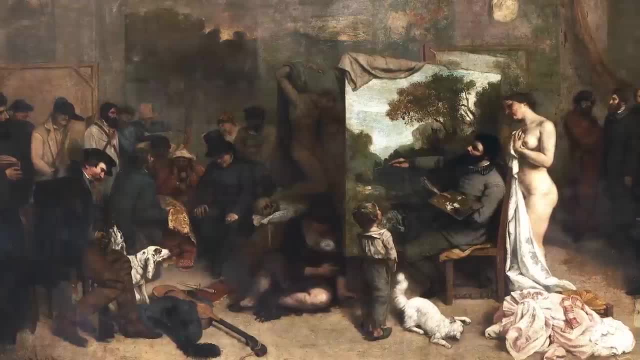 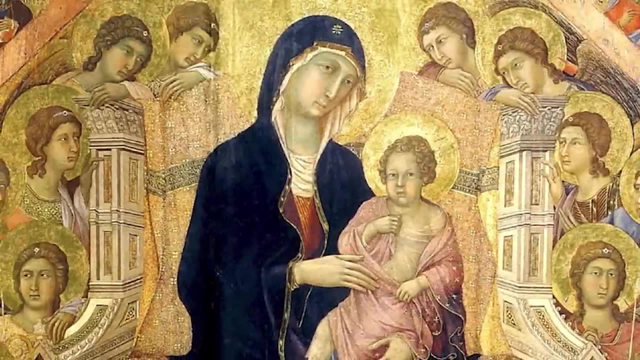 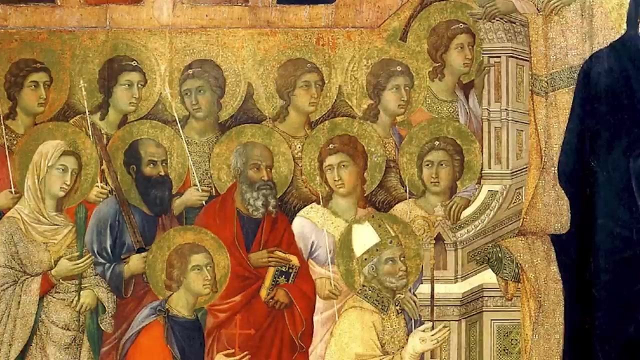 parts of a composition, like landscape backgrounds. If you were to take almost any painting from a Renaissance workshop, you would find it collaborative. In such situations, the master would paint the more central figures or faces, while the apprentices would be tasked with imitating the master's style in completing the rest of the painting, As witnessed in. 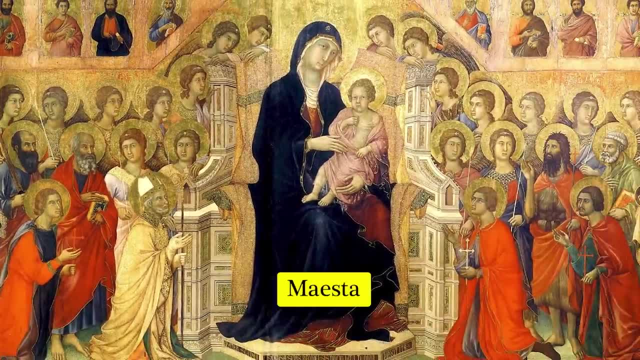 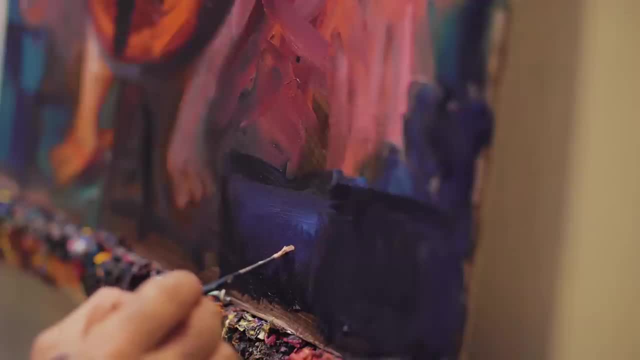 Duccio's most famous altarpiece, Maestà. While contracts occasionally specified that the master should execute certain parts of a composition, guild rules allowed the master to sign any work from their shop as their own. So even if an apprentice did the majority of the work, the master would sign his own.